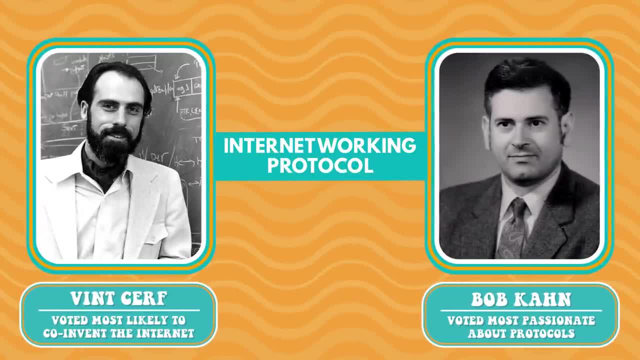 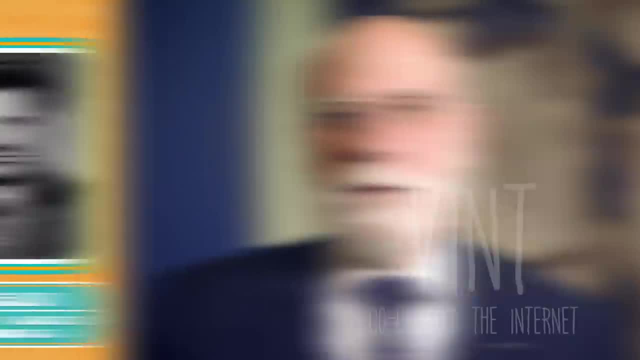 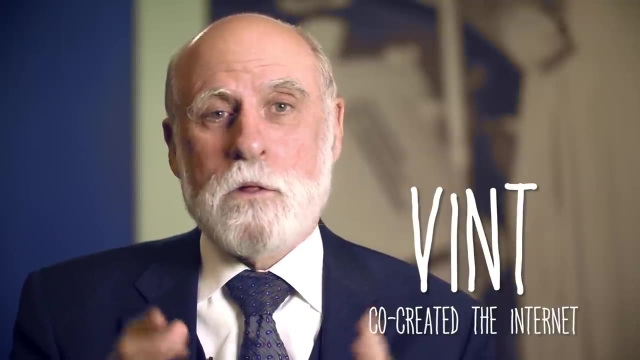 Bob Kahn to invent the internetworking protocol to make communication possible. This invention laid the groundwork for what we now call the internet. The internet is a network of networks. It links billions of devices together all around the globe. So maybe you're connected with a laptop or a phone through Wi-Fi, But then 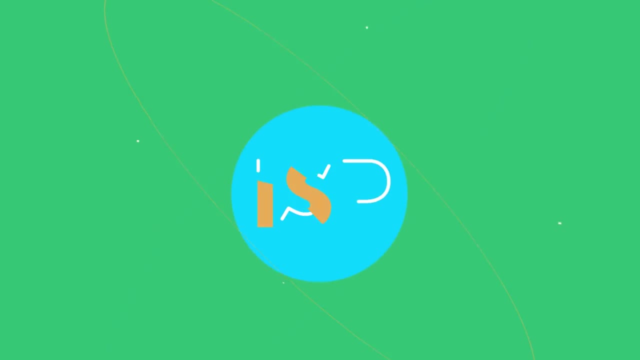 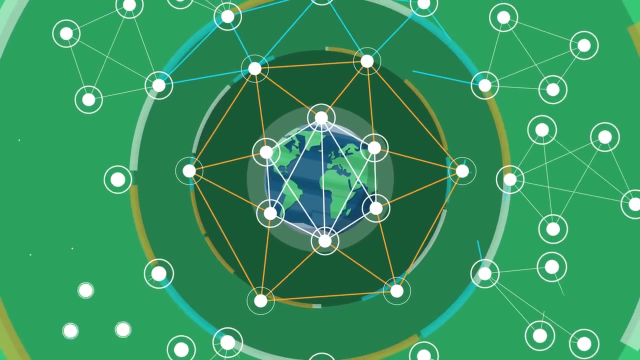 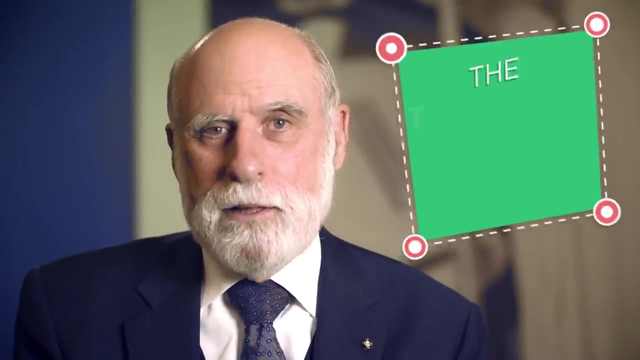 that Wi-Fi connection connects to an internet service provider, or ISP, and that ISP connects you to billions and billions of devices around the world through hundreds of thousands of networks that are all interconnected. One thing that most people do not appreciate is that the internet is really a design philosophy. 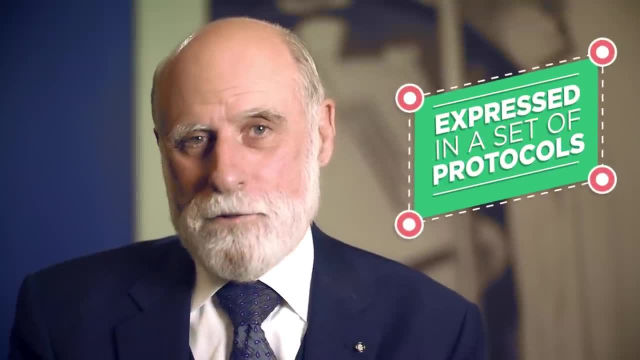 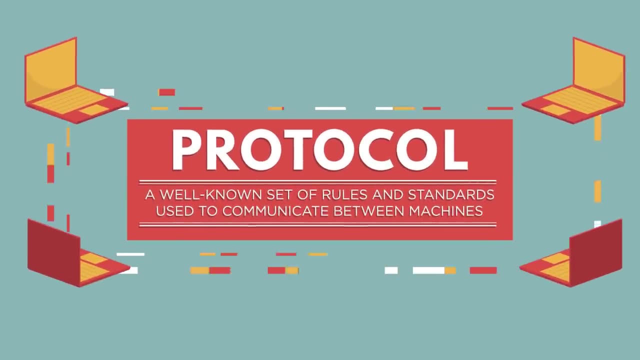 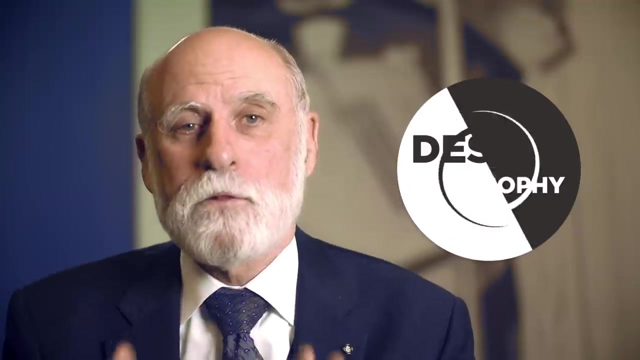 and an architecture expressed in a set of protocols. A protocol is a well-known set of rules and standards that, if all parties agree to use, it, will allow them to communicate without trouble. The fact that the internet works is less important than the fact that this design philosophy 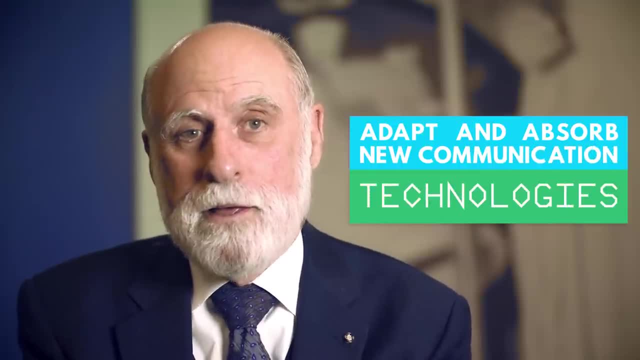 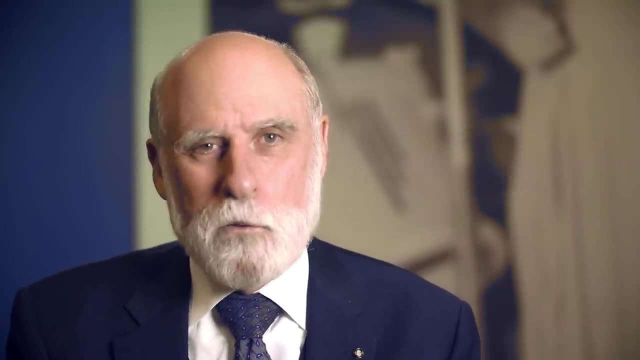 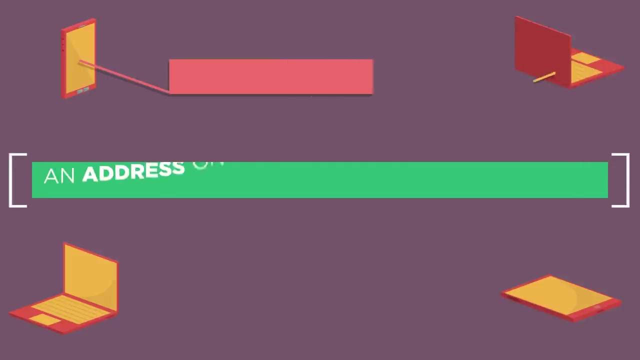 has allowed the internet to adapt and absorb new communication technologies. This is because, in order for a new technology to use the internet in some fashion, it just needs to know which protocols to work with. All the different devices on the internet have unique addresses- An address on the internet. 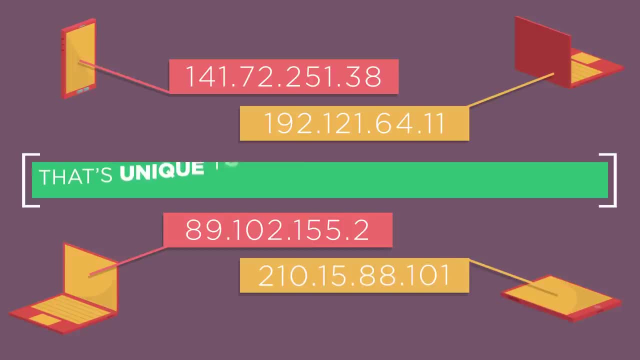 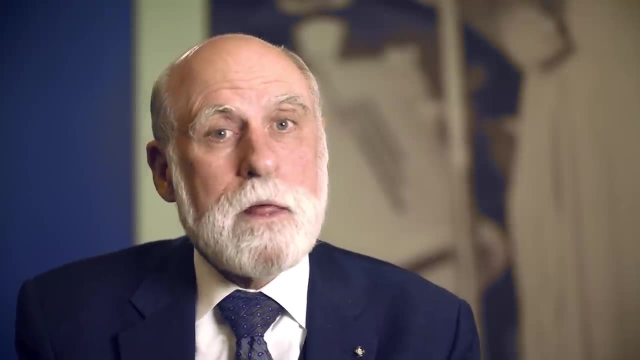 is just a number similar to a phone number or a sort of street address that's unique to each computer or device at the edge of the internet. This is similar to how most homes and businesses have a mailing address. You don't need to. 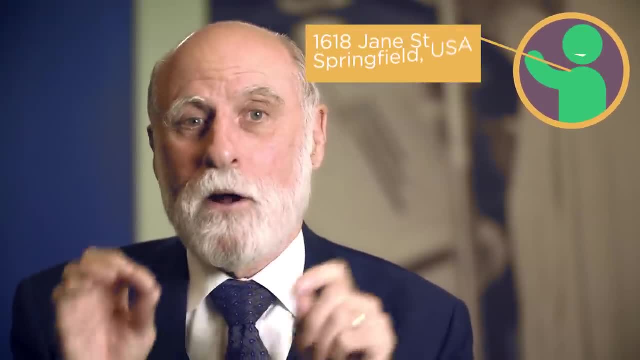 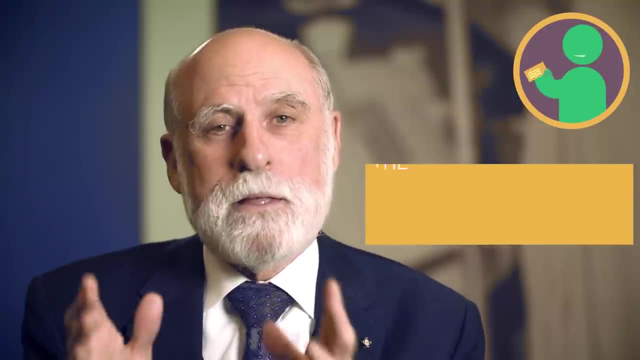 know a person to send them a letter in the mail, but you do need to know their address and how to write the address properly so the letter can be carried by the mail system to its destination. The addressing system for computers on the internet is similar and it forms part of. 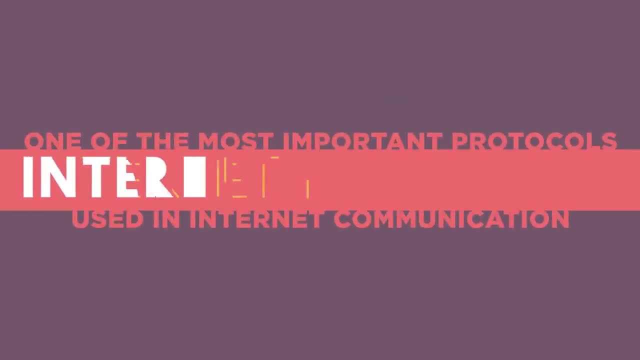 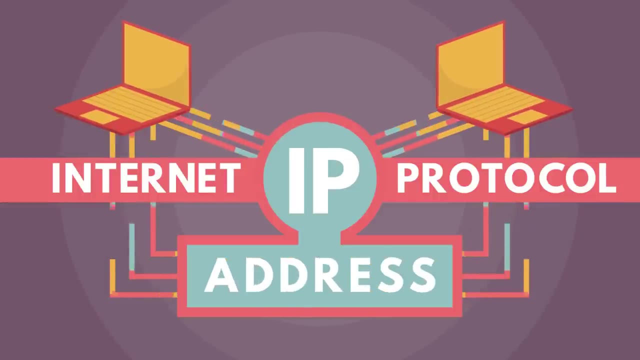 one of the most important protocols used in internet communication, simply called the Internet Protocol or IP. A computer's address, then, is called its IP address. Visiting a website is really just your computer. asking another computer for information, Your computer sends a message. 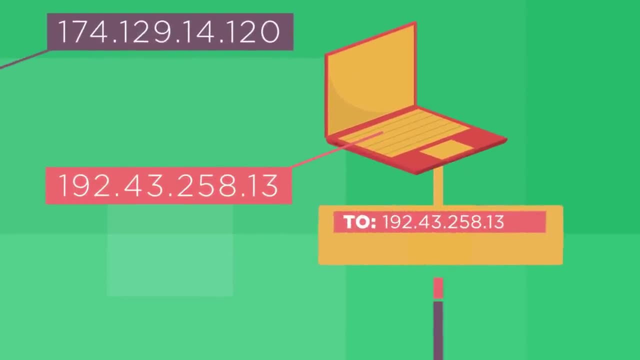 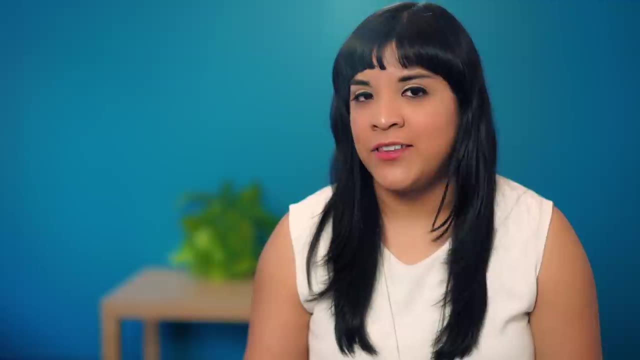 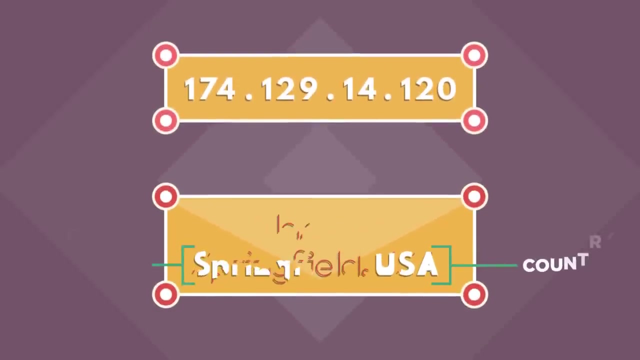 to the other computer's IP address and it also sends along its origin address, so the other computer knows where to send its response. You may have seen an IP address. It's just a bunch of numbers. These numbers are organized in a hierarchy, Just like a home address has a country a. 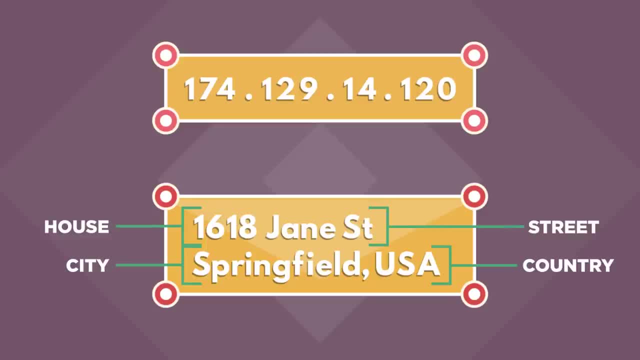 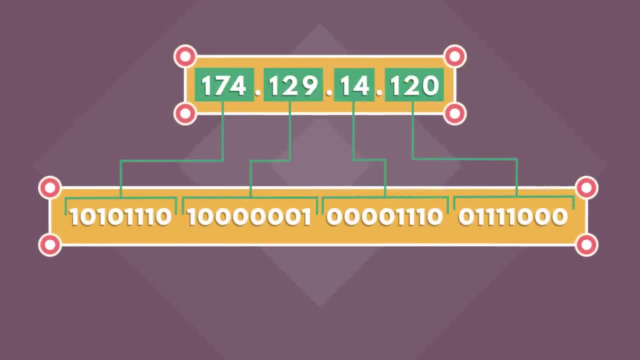 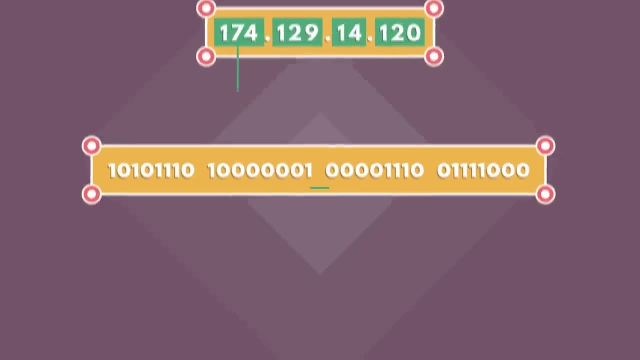 a street and a house number. an IP address has many parts, Just like all digital data. each of these numbers is represented in bits. Traditional IP addresses are 32 bits long, with 8 bits for each part of the address. The earlier numbers usually identify the country and regional network of the device. 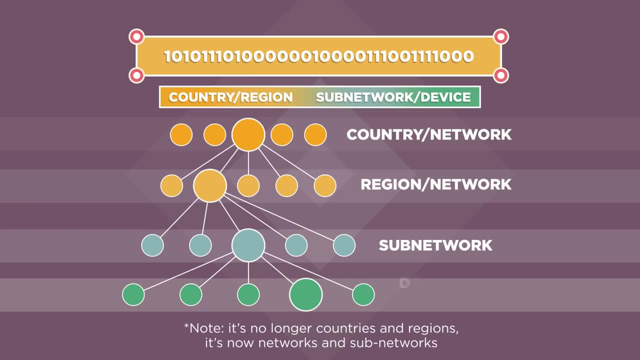 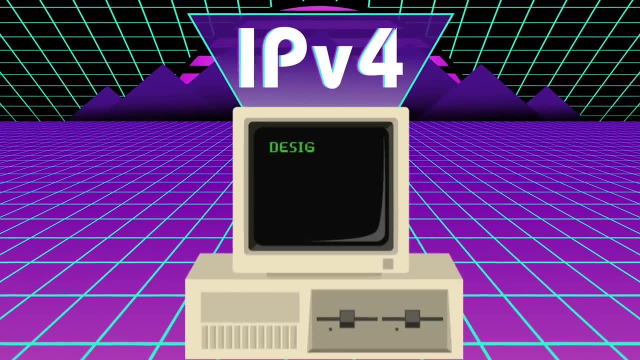 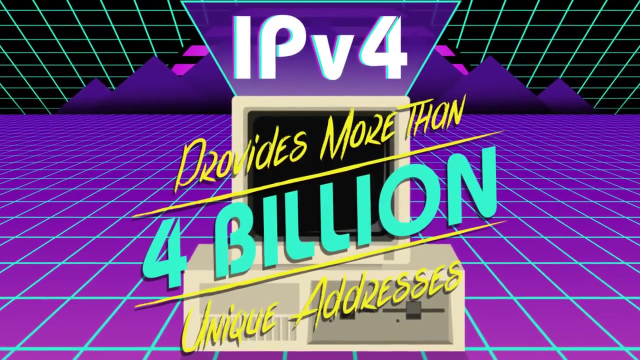 Then come the sub-networks and then finally, the address of the specific device. This version of IP addressing is called IPv4. It was designed in 1973 and widely adopted in the early 80s, and provides for more than 4 billion unique addresses for devices connecting to the Internet. 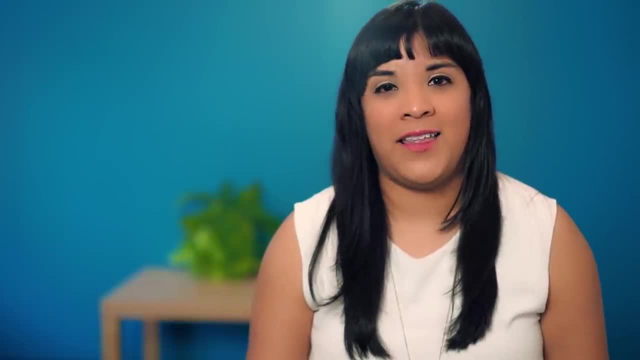 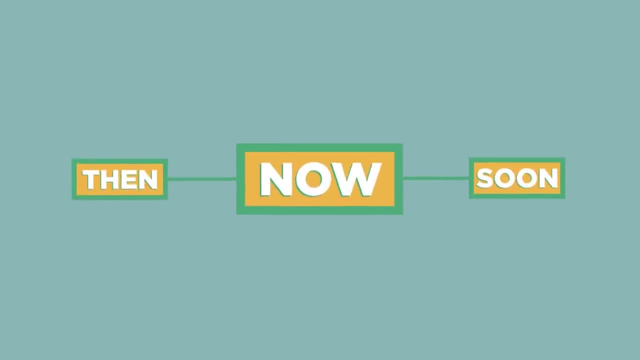 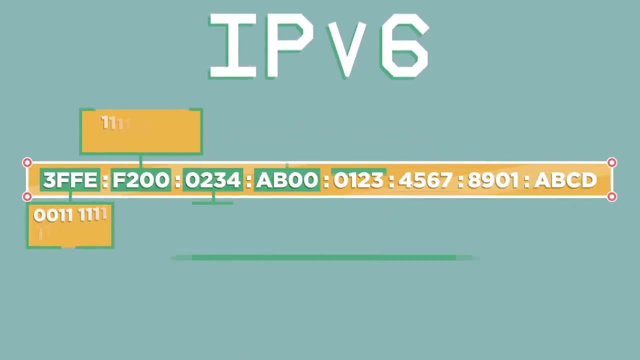 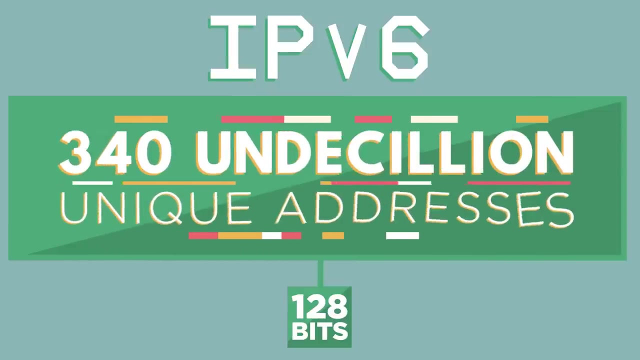 But the Internet has turned out to be much more popular than even Venn's surf imagined, and 4 billion unique addresses won't be enough. We're now in the middle of a multi-year transition to a longer IP address format Called IPv6,, which uses 128 bits per address and provides over 340 undecillion unique addresses. 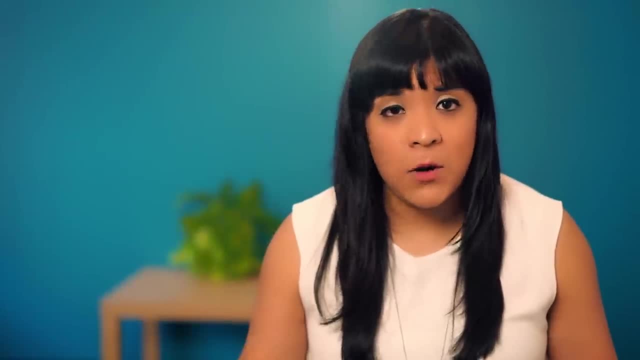 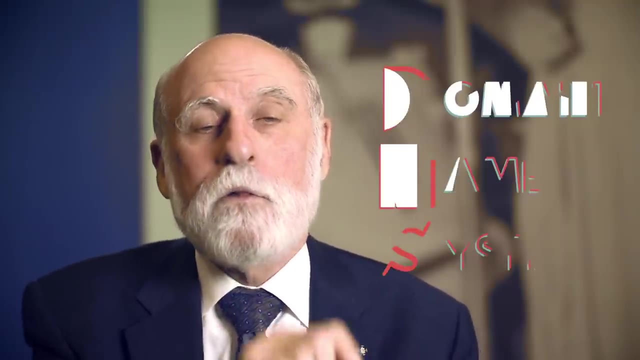 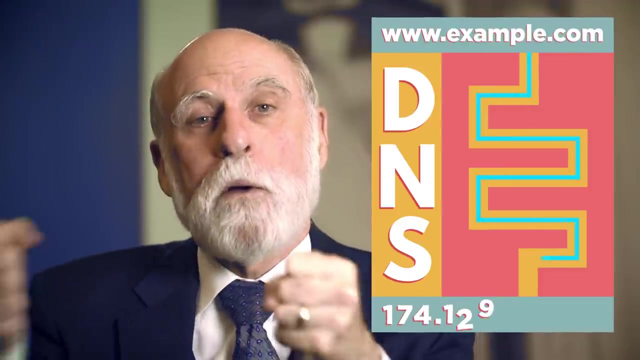 That's more than enough for every grain of sand on earth to have its own IP address. Most users never see or care about Internet addresses. A system called the Domain Name System, or DNS, associates names like wwwexamplecom with the corresponding addresses. 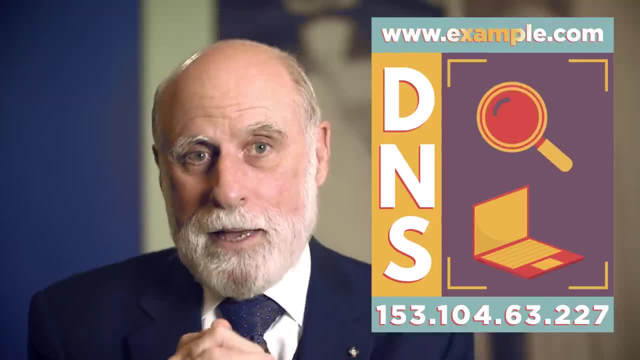 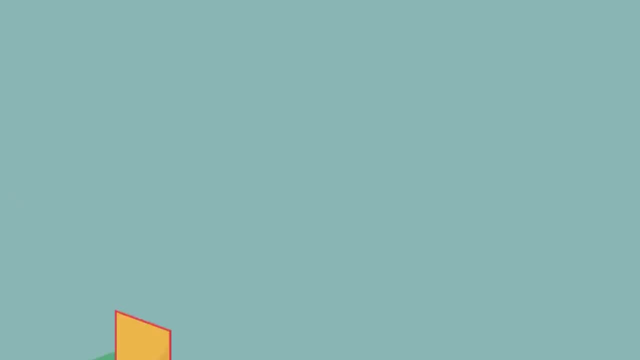 Your computer uses the DNS to look up domain names and get the associated IP address, which is used to connect your computer to the destination on the Internet, And it goes a little something like this: Hey, hi there, I want to go to wwwcodeorg. 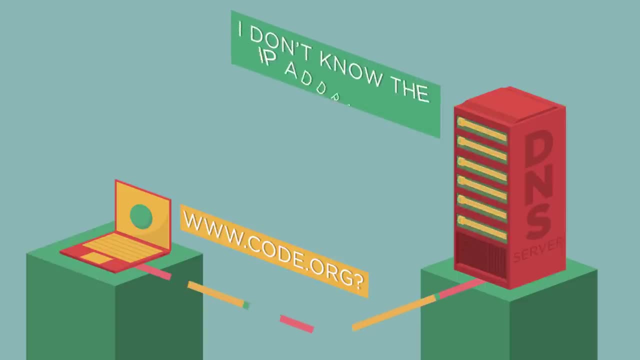 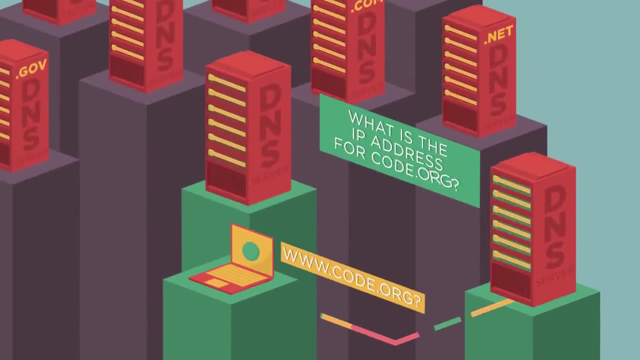 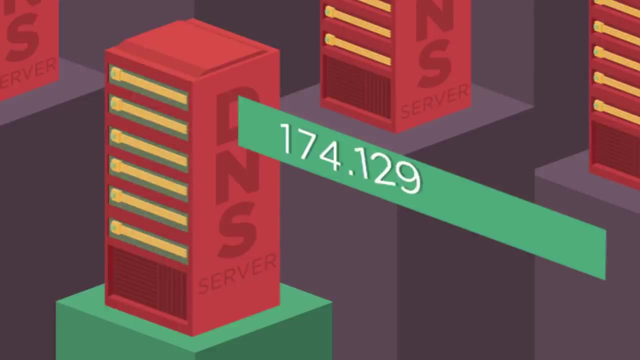 Mmm, yeah, I don't know the IP address for that domain. Let me ask around, Hey, Hey, you know how to get to codeorg. Nope, Yeah, I got it right here. It's 174.129.14.120..